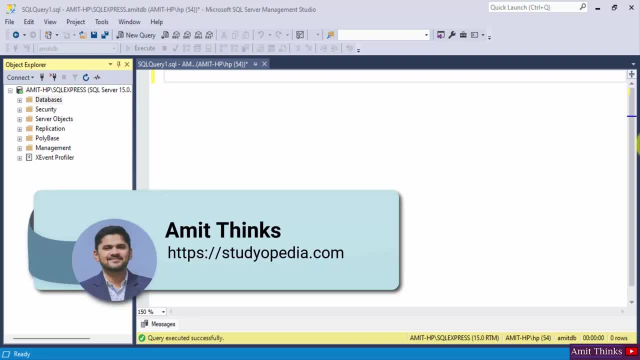 Hello guys, welcome to Amit things. In this video we will see how we can easily work with a create index statement to create indexes in SQL. So basically, indexes are used to retrieve data from a database faster than any other way. Let's see how we can create. 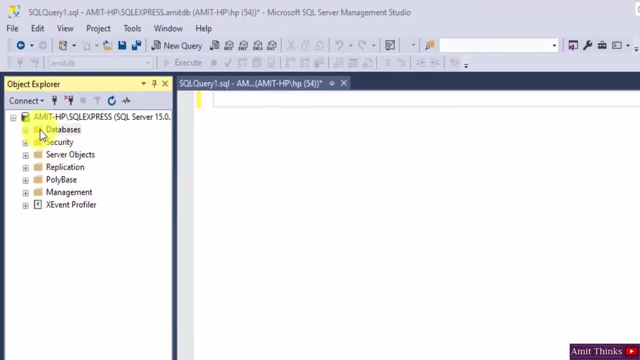 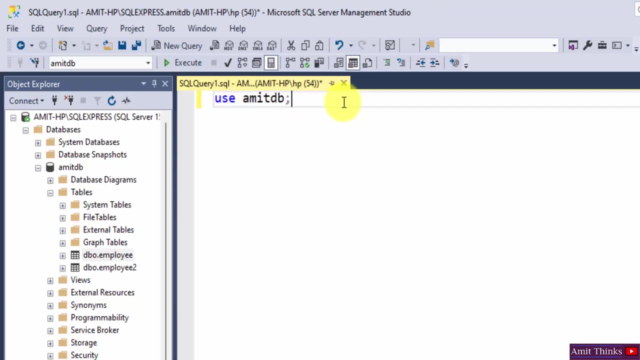 an index quickly. We will see a live example here. and we have a database, Amit DB, Within that we have a table employee. So let's see, Let's enter the database Amit DB using the use command. Here it is. Now let us see the records of the employee table using select. 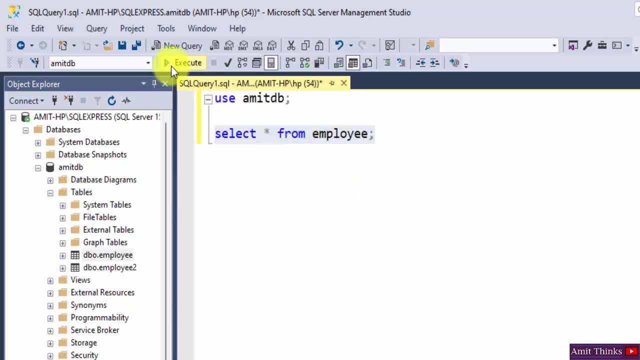 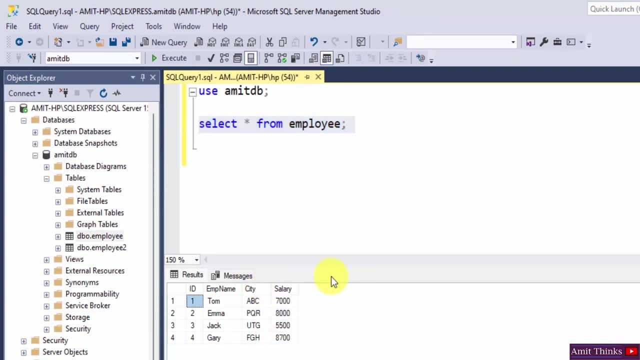 star from employee: Select and execute. So here you can see, the following are records. Okay, so we will create an index using it. How, Using the create index statement? Let us use the command Create index, Add the name of the index. Let's say, I'll add my index, the name On command. 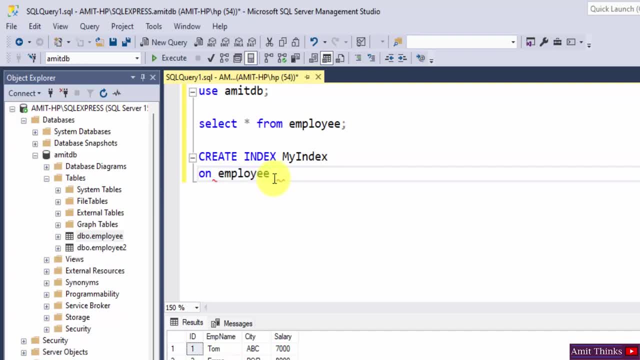 On. now mention the table name. that is, our table name is employee and brackets. under brackets, you will be adding the column name, that is. this statement will create an index, named my index, on the column which we will add here. Let's say, I'll add EMP name, Okay. 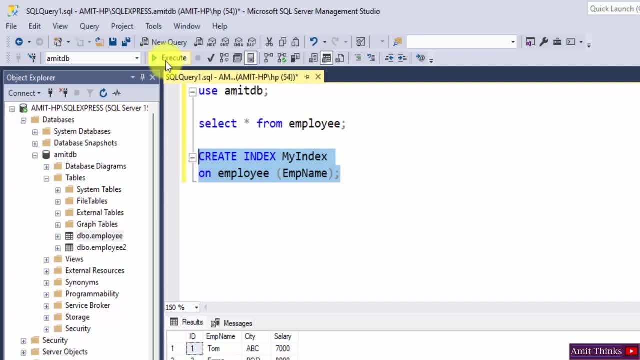 Semicolon and let's run it. So I ran it and command completed successfully. You need to remember that the users can never see the indexes, but they are only used to speed up the searches, that is, speed up the queries. Now we can also create indexes with a list. 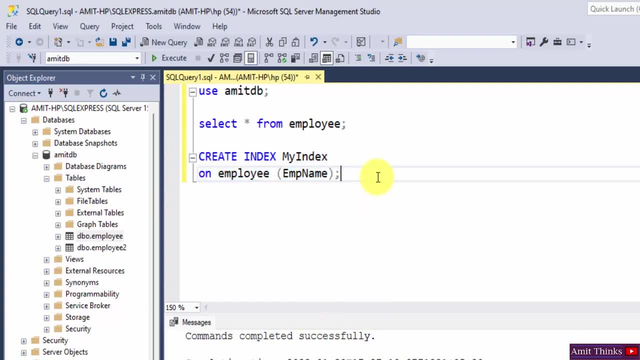 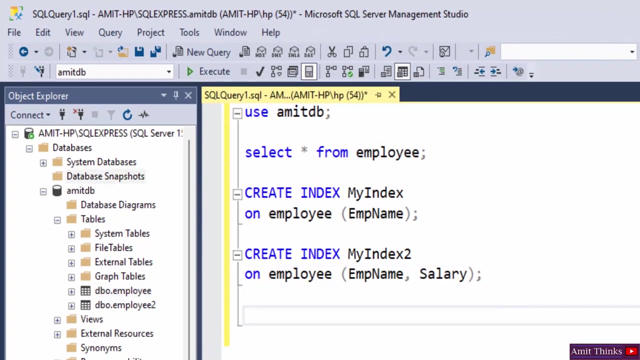 of column names, that is, using combination of columns. How, Let me use this name? or second index, my index to, and I'll add multiple columns in it. Okay, salary. Okay, now I'll execute it. The second index completed successfully. command completed successfully. Okay, guys, so we created two indexes. So, guys, now let us delete.